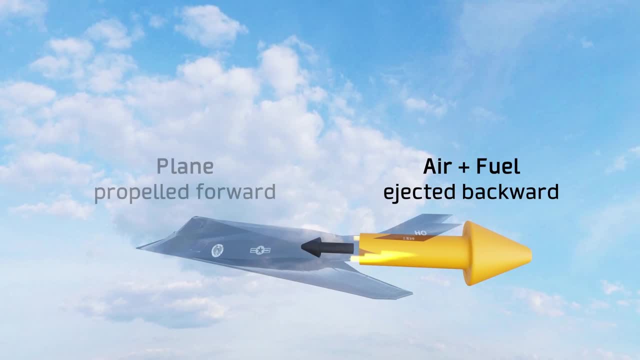 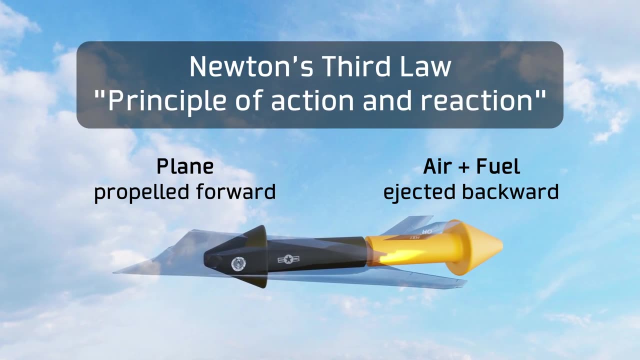 When a force is exerted on an object- a force of equal intensity but opposite direction- is exerted on the object that produced it. This is better known as Newton's third law, or the principle of action and reaction. Understanding this, there is a technology that takes this. 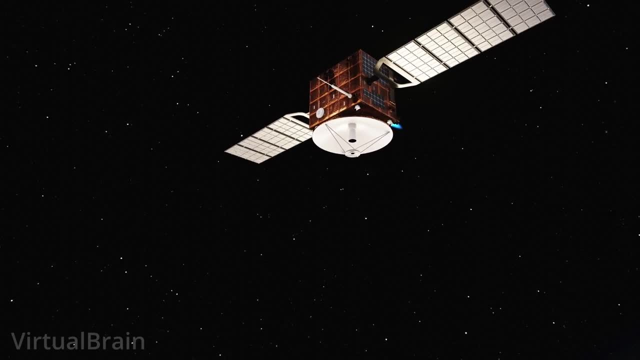 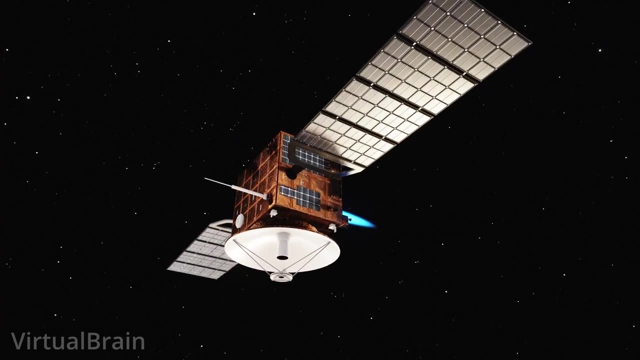 concept to the extreme, reducing the amount of propellant but ejecting it at speeds of even hundreds of kilometers per second. I am talking about electric propulsion systems, of which there are several types, the most widely used today being ion thrusters and Hall thrusters. 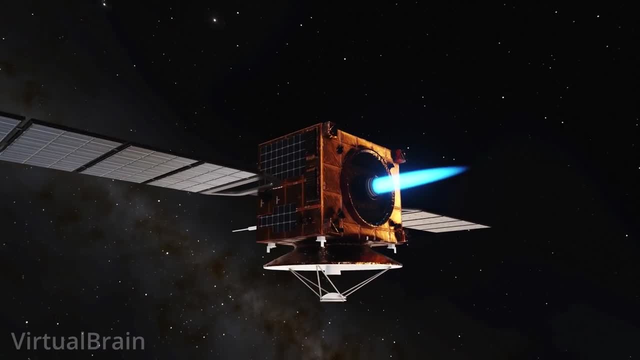 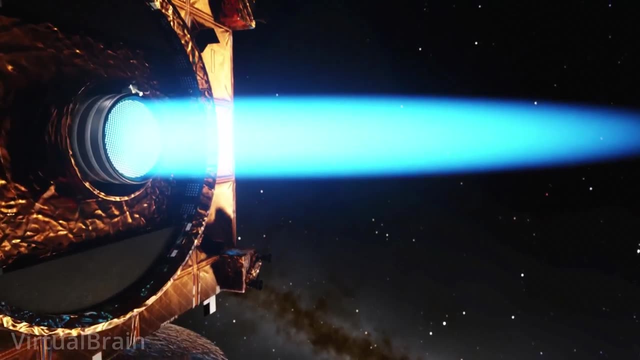 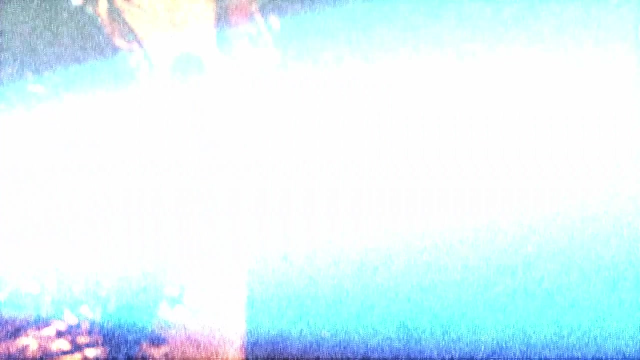 In simple terms, they use electric fields to accelerate atoms and eject them at high speeds, But obviously there is much more to it. So in this video, we will look at how an ion thruster works, in addition to its benefits, limitations and uses. To understand how an ion thruster works: 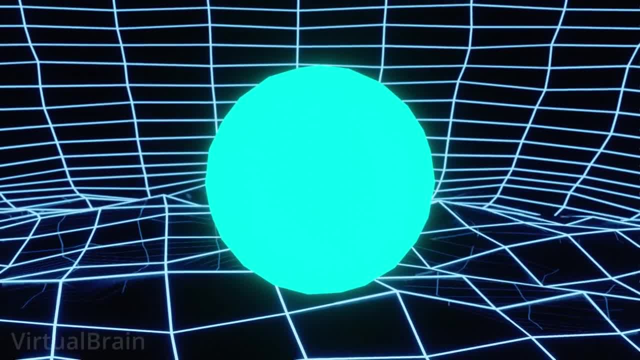 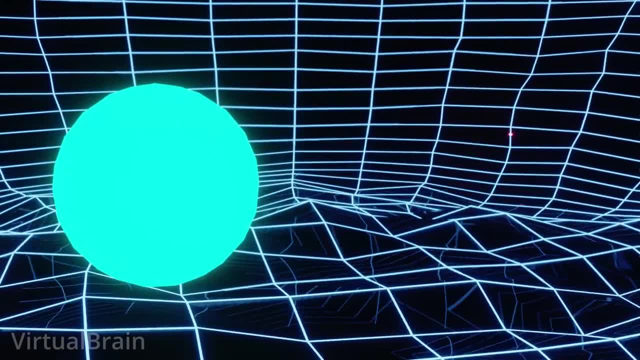 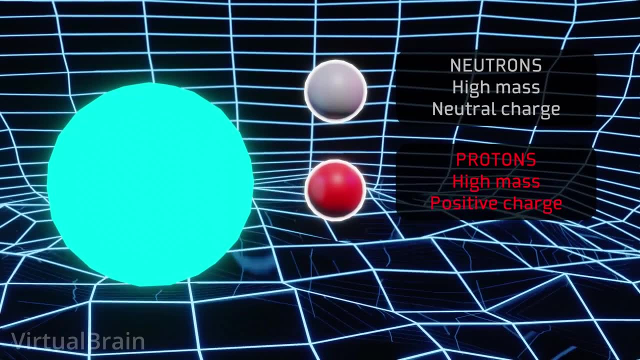 we must first understand how atoms are composed, what an ion is and what plasma is. An atom, in simple terms, is composed mainly of three subatomic particles: Neutrons, which have a high mass but no electric charge. Protons, also of high mass, but with a positive charge. 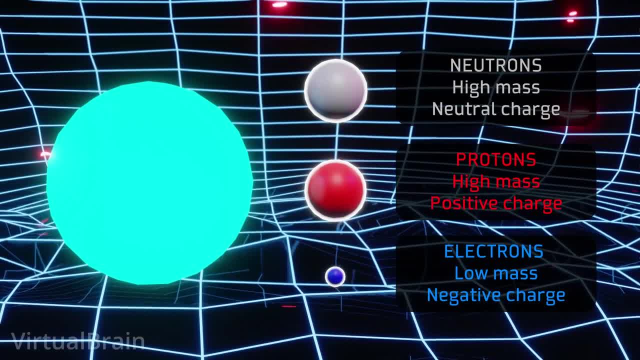 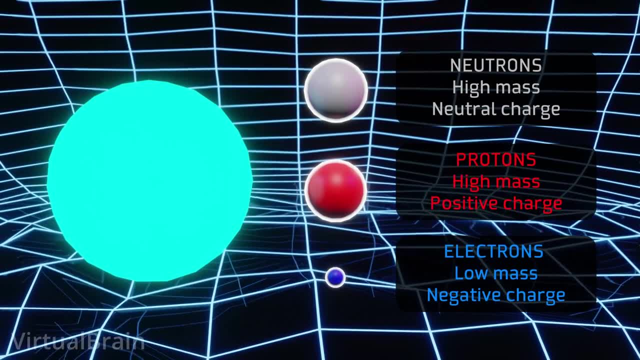 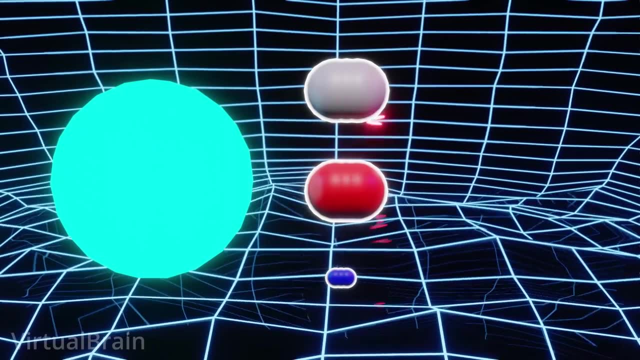 And electrons with a low mass and a charge of equal value to that of the proton, but negative In this case. when I say high or low mass, I mean in relative terms, with electrons having a mass about 1,800 times smaller than protons or neutrons. Understanding this, the atoms of 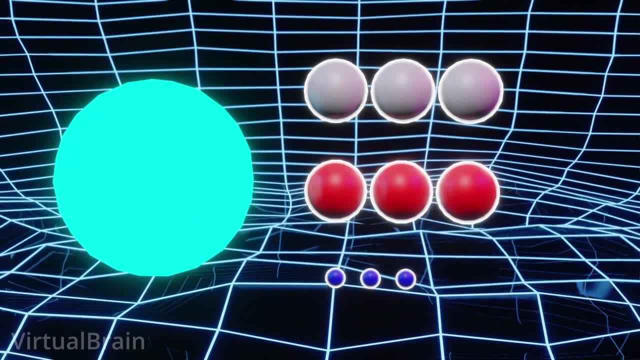 different elements are composed of different amounts of these particles and as long as the amount of protons is equal to the amount of electrons, the atoms of different elements are equal to the amount of neutrons. the charges cancel out and the atom will have a neutral charge. 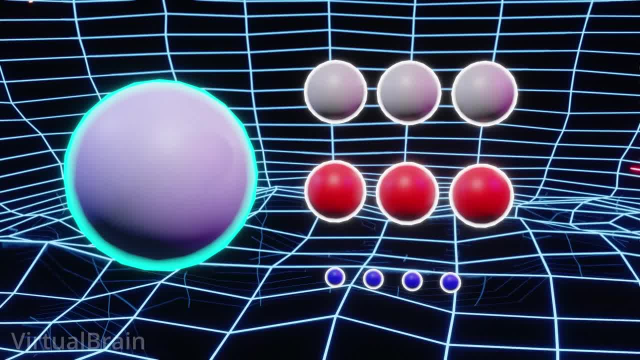 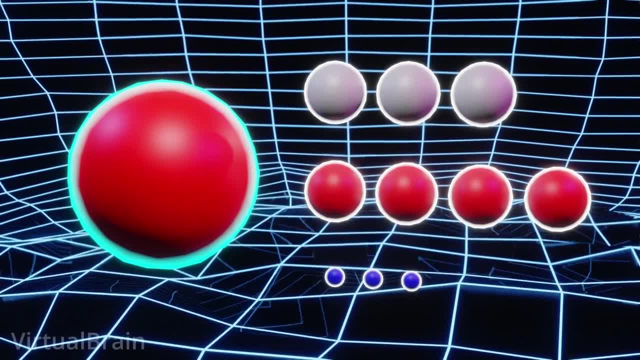 On the other hand, if there are more electrons than protons, the atom will have a negative charge, and if there are more protons than electrons, the atom will have a positive charge. These two cases are what is known as an ion. 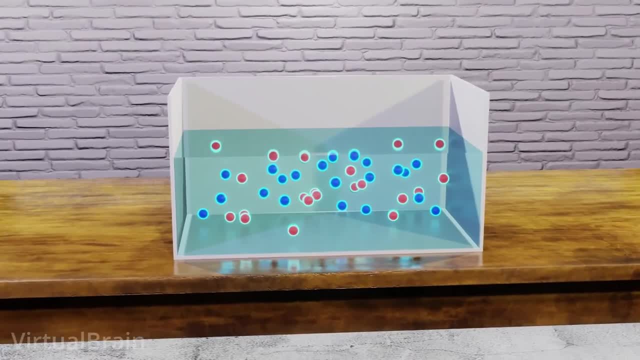 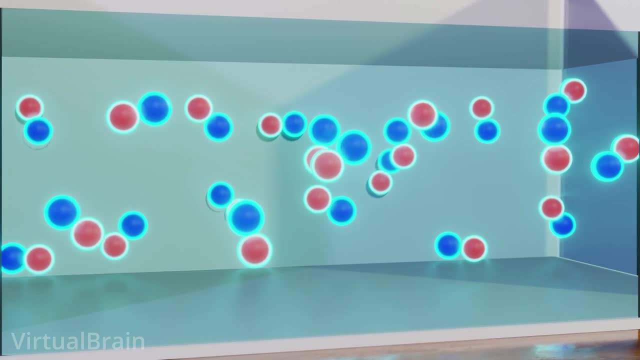 Under normal conditions, if we had a liquid or a gas with a mixture of ions with different charges, they would interact with each other, attracting each other if they have electric charges of opposite signs. This is why, in the process of the ionization process, new molecules are formed with different 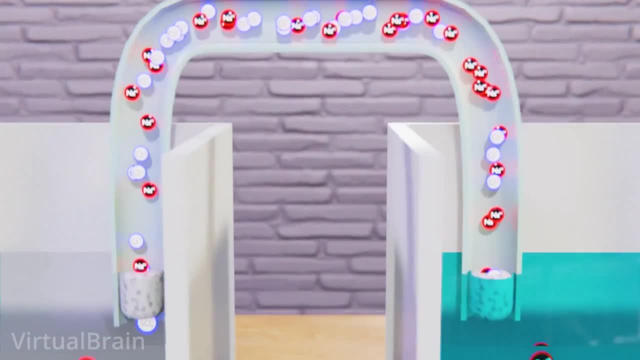 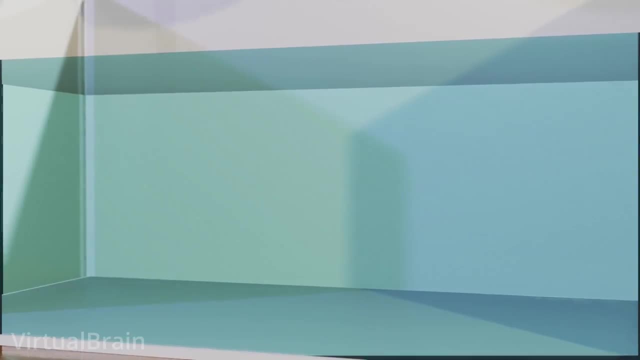 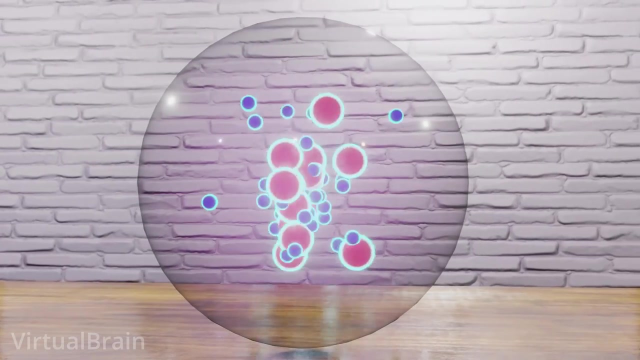 properties similar to what we saw in the video on how batteries work, But all this behavior changes slightly when the ions are in a state of matter known as plasma, in which the ions and electrons will remain separated, which also allows them to act as 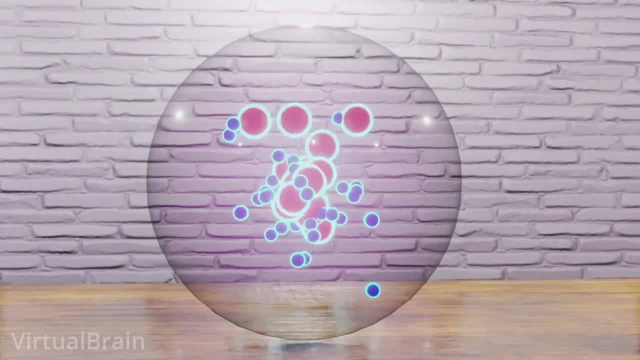 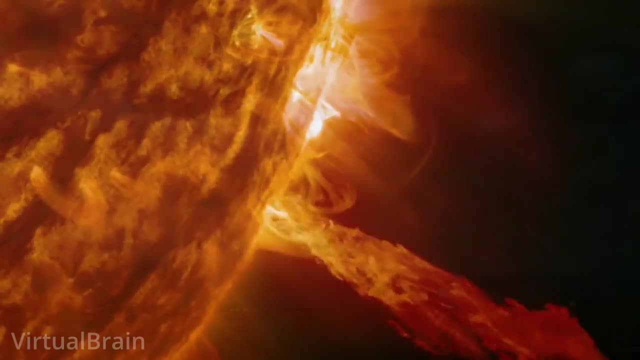 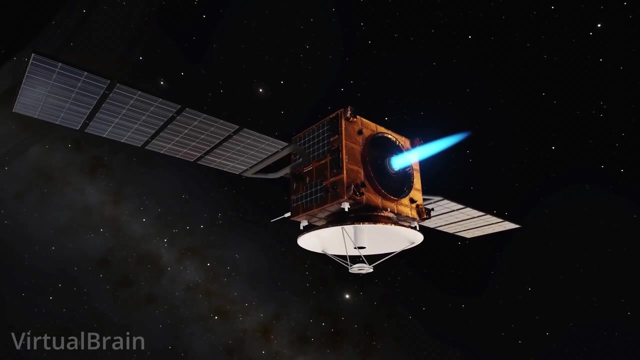 electrical conductors, Although it is important to mention that for this to happen, some conditions must usually be met, such as high temperatures, strong electromagnetic fields or the presence of microwaves. Getting that out of the way, let's look at how to build an ion thruster and the effect each of 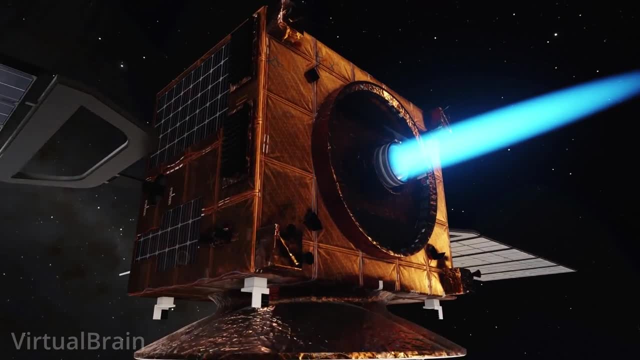 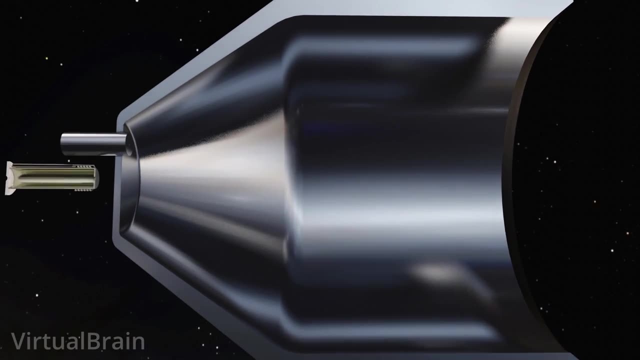 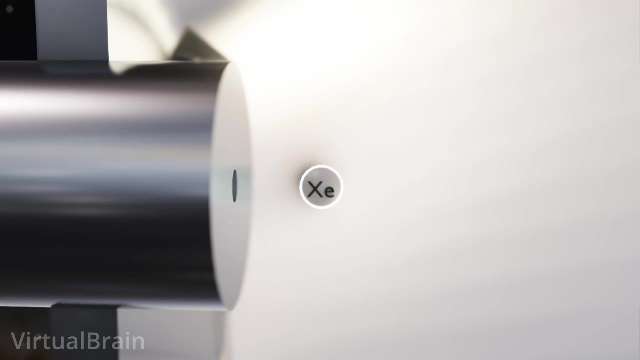 its components has. The first element we will need is a container with an open end and a closed end To this. we will add an inlet at the closed end through which we will introduce a gas such as xenon, which is a noble gas, That is to say that in normal conditions, it is presented as 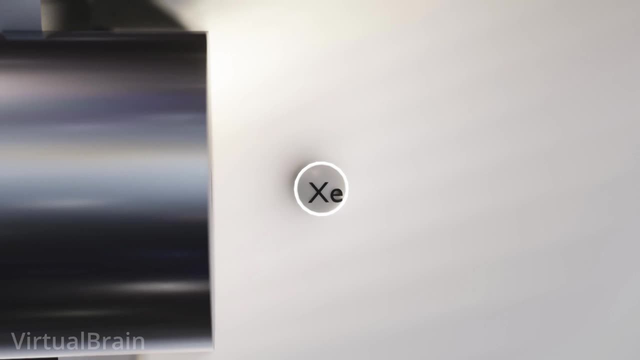 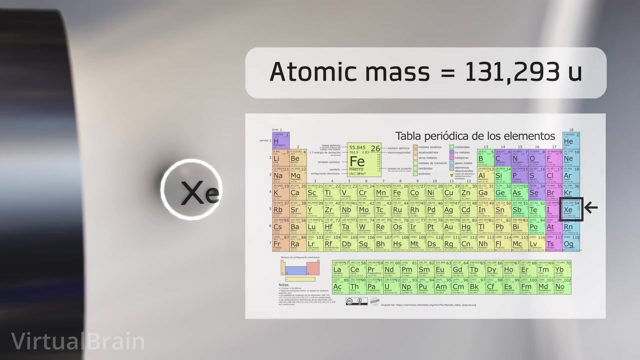 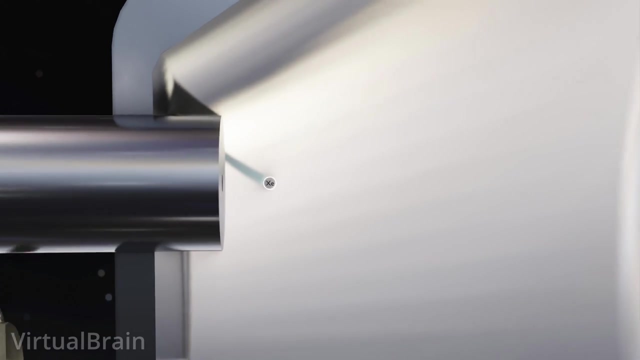 individual atoms with neutral charge, which does not react easily with other elements and therefore facilitates the handling and storage. But, more important than that, it is an element with a high atomic mass which, as we will see later, is extremely important for the operation of the 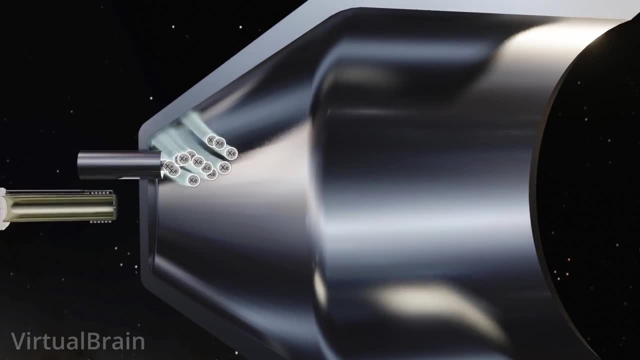 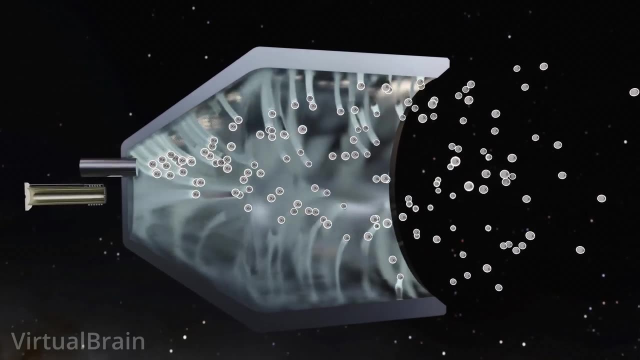 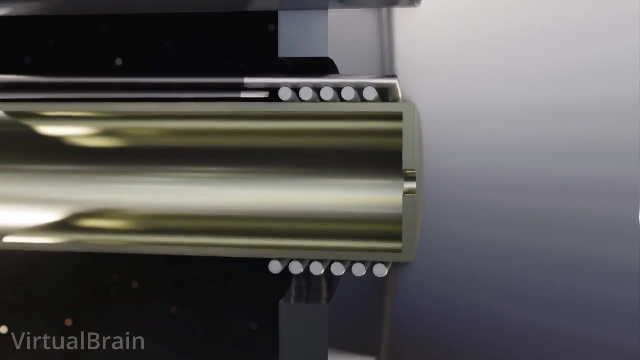 propellant. At this point, if we let the xenon in, nothing will happen. it will simply disappear. The next element we will add will be an electron gun, also known as a hollow cathode. This consists of a tube with a hole which inside has a material, such as tungsten, covered with. 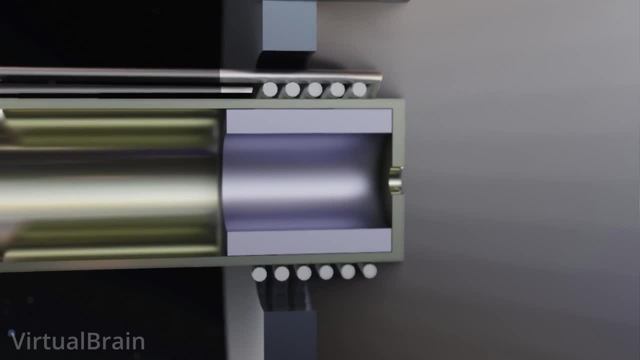 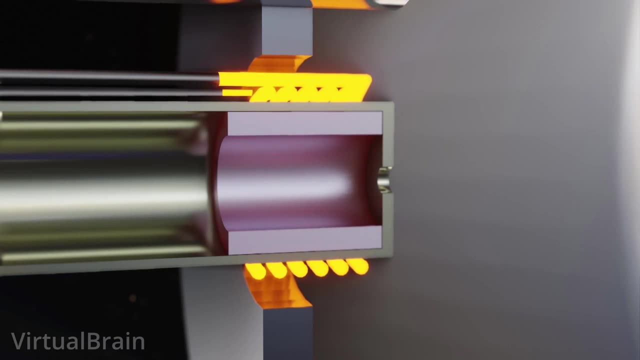 barium oxide, which is also surrounded by a resistor. The principle of its operation is that, by heating the resistance, this will heat the material inside which, by a phenomenon known as thermionic emission, will begin to emit a gas. This will heat the material inside which, by a 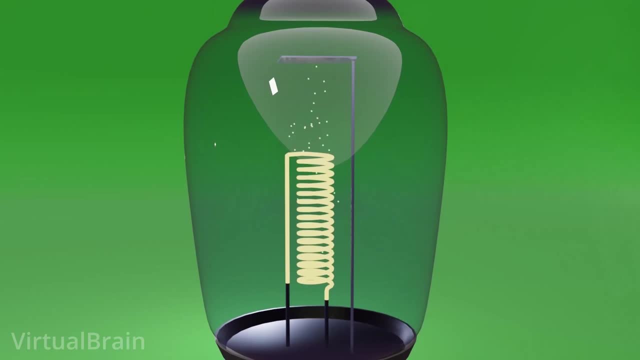 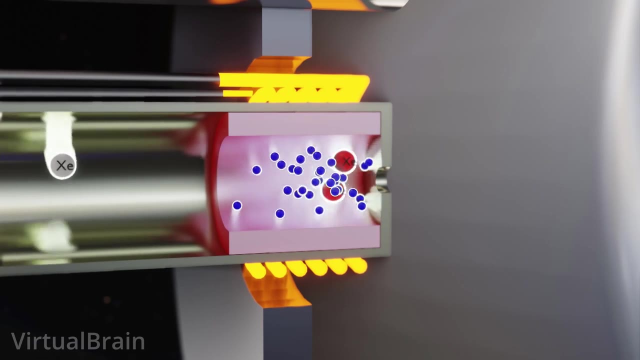 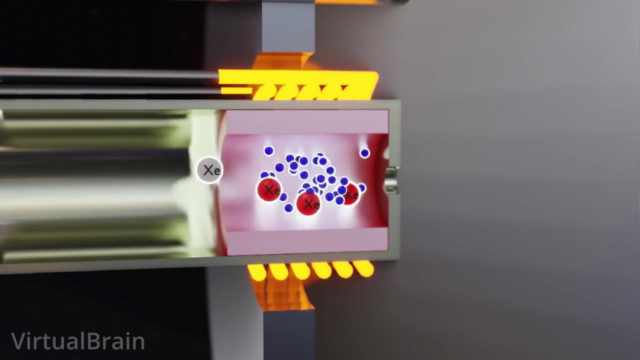 phenomenon known as thermionic emission will begin to emit electrons, similar to how vacuum diodes work. A small amount of xenon is then injected into the tube from the rear. Having a small volume at high temperature, with electrons being continuously emitted, generates the correct environment for plasma to be created, More specifically, the electrons. 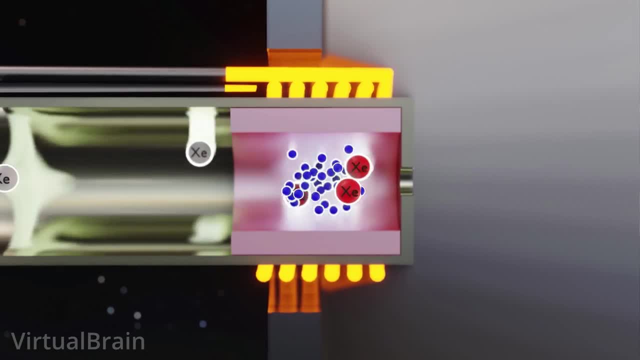 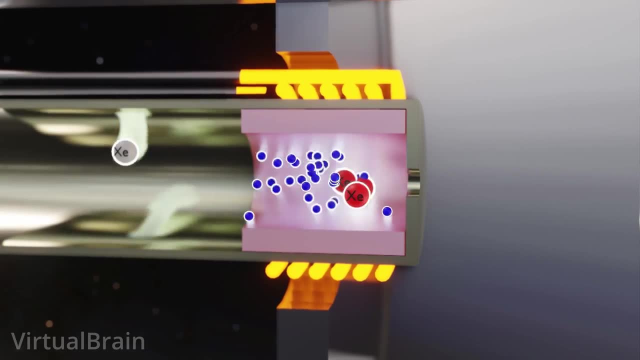 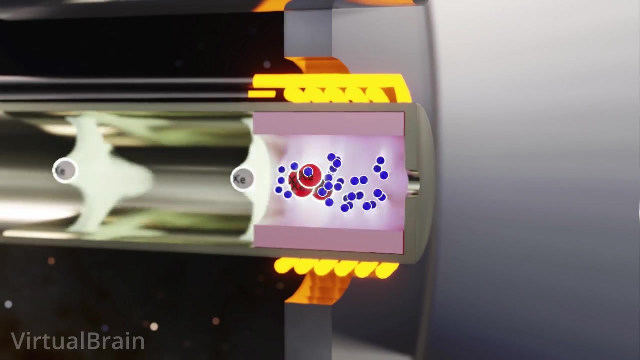 collide with the xenon atoms which, let's remember, had a neutral charge and caused them to lose one of their electrons. Now we will have a plasma volume composed mostly of electrons and since xenon continues to be injected from the rear, it will be forced out through the hole. Furthermore, to aid this, 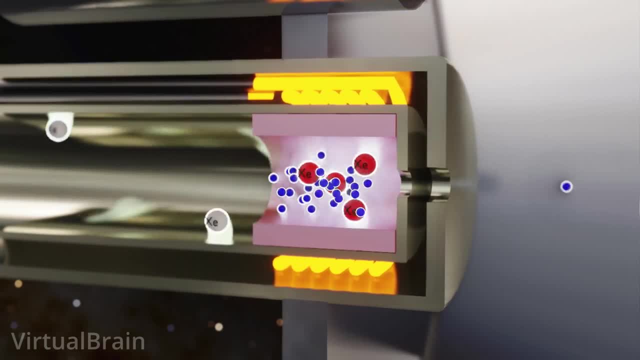 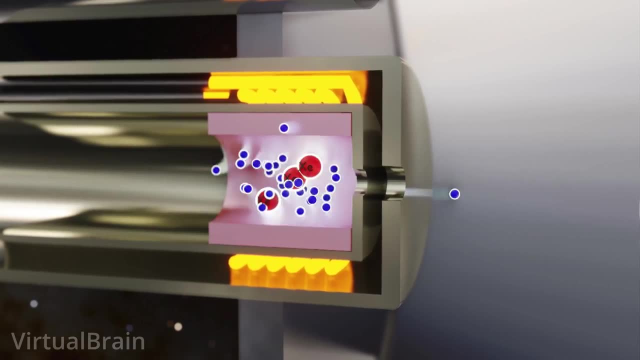 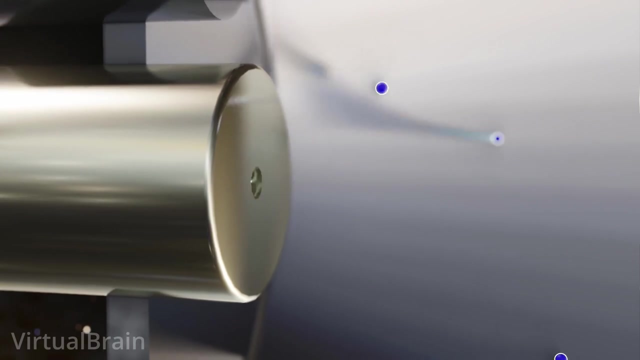 process, a positively charged cover is added which has a dual function: Firstly, it guides the electrons into the orifice and secondly, it prevents other particles from entering the section where the plasma is generated and affecting its operation. If we reanalyze the components we have so far and inject xenon into the main container at the same, 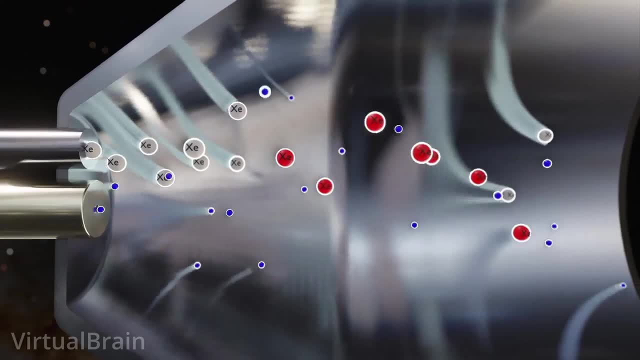 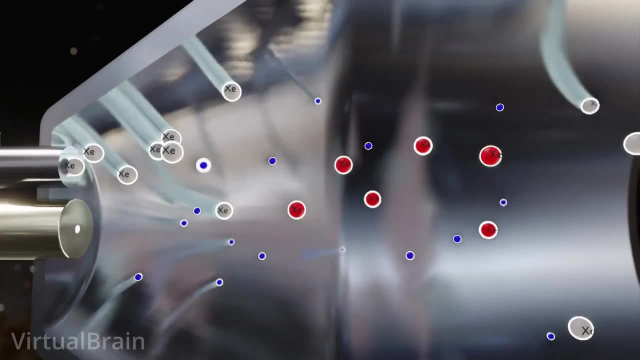 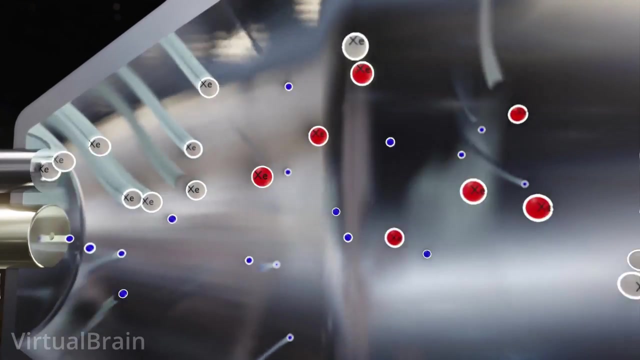 time we use the electron gun, the behavior will be repeated, but this time on a larger scale. Again, the electrons collide with the neutral xenon. they will remove one of its electrons and convert it into positive ions, generating plasma. However, this time the conditions will. 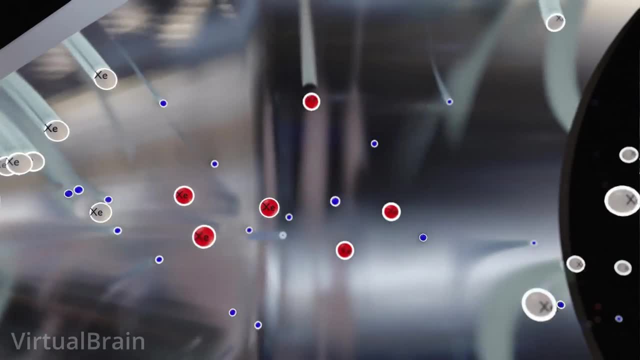 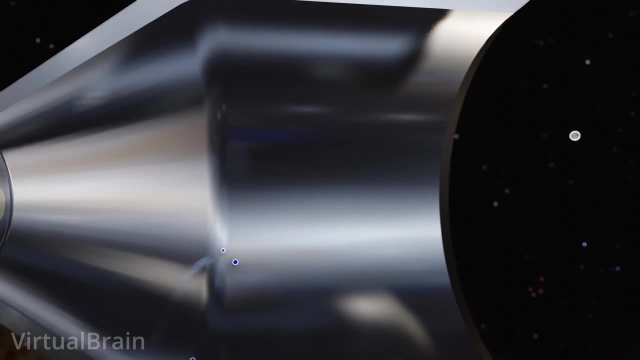 be different in terms of pressure, temperature and magnetic fields present. This time, when the hydrogen ionizer generates a positive ion, it will not be able to achieve its desired effect. However, this time, the ionizer will also receive positive ions, which will increase the efficiency. 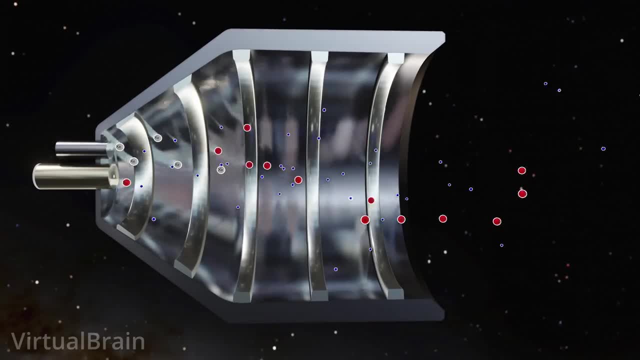 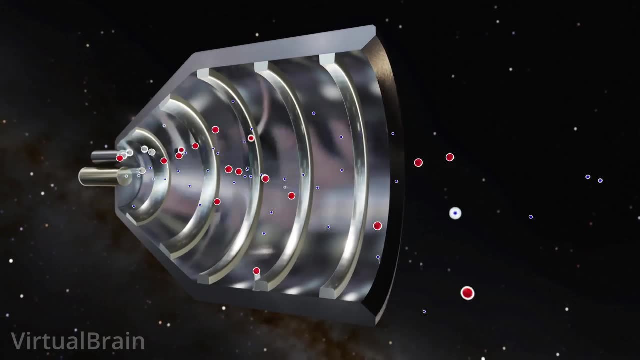 of the paste, and this amount of ionization will not be very efficient. To overcome this, a series of magnetic rings are added around the main container, which increase the efficiency of ionization and help contain the generated plasma. Having a continuous source of large amounts of plasma, we can finally start talking about how the propulsion is generated. For this purpose, a double grid is added to the open end of the container, each of them electrically charged due to the application of the new project force. 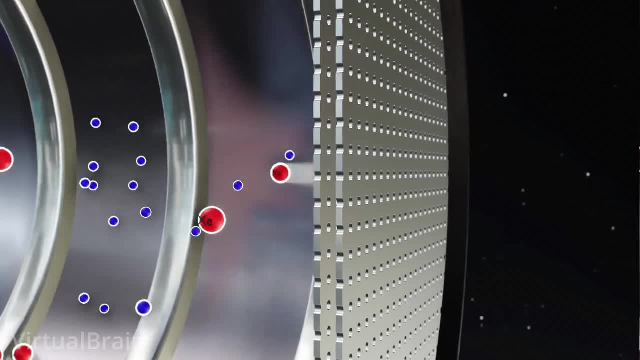 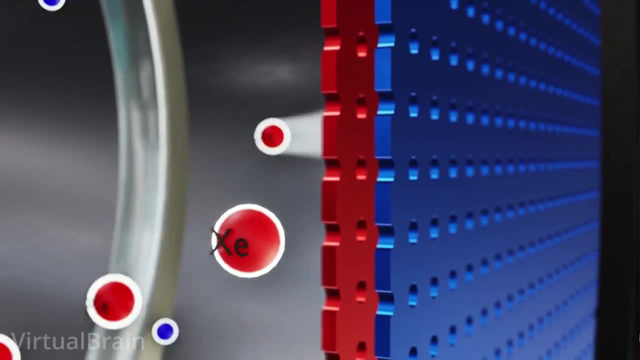 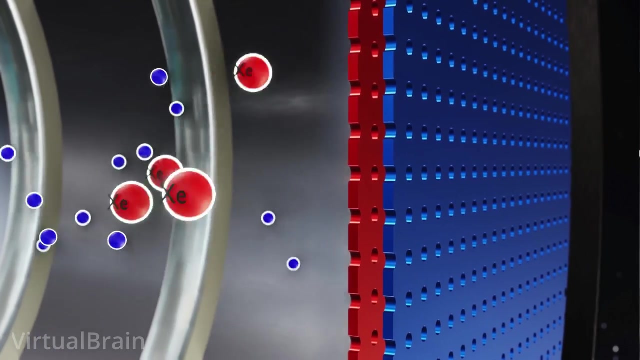 charged due to the application of high voltages. The inner one is positively charged and the outer one negatively charged. Since plasma is continuously being generated, the pressure inside the container will be increasing and since these grids are the only way out- both electrons and xenon ions- 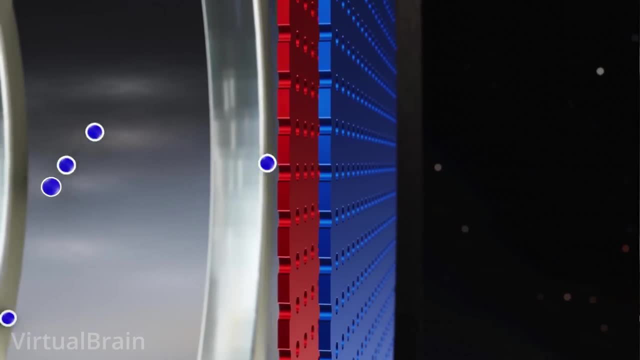 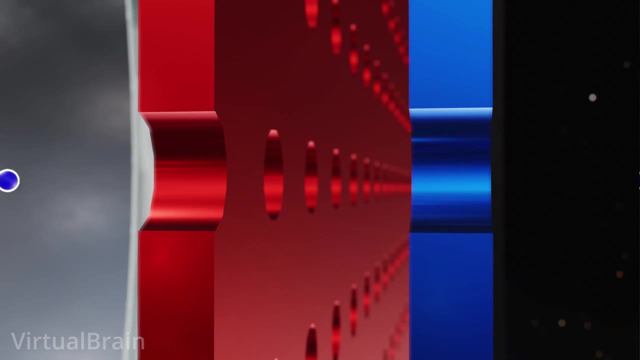 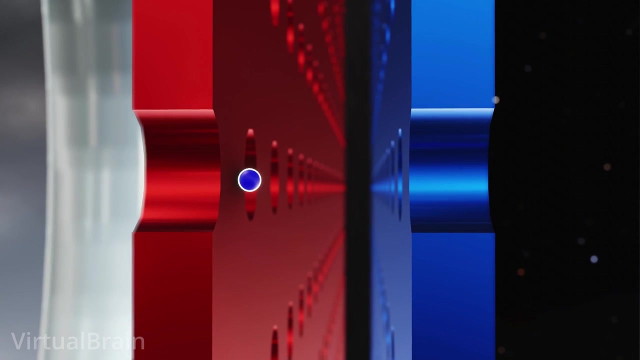 will try to pass through them. If we analyze the behavior of an electron, it will be attracted to the positively charged inner grid and may even pass through due to the pressure inside the container. But since the second grid is negative, the electron will be repelled, pushing it back. 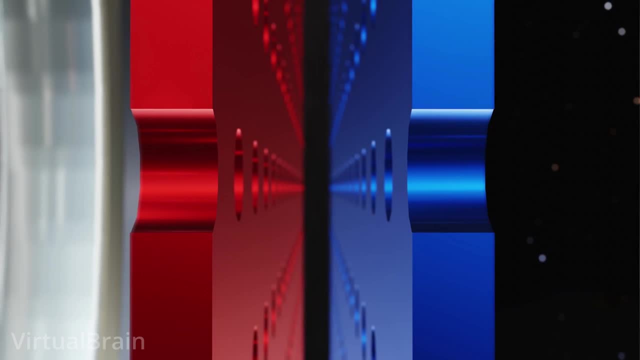 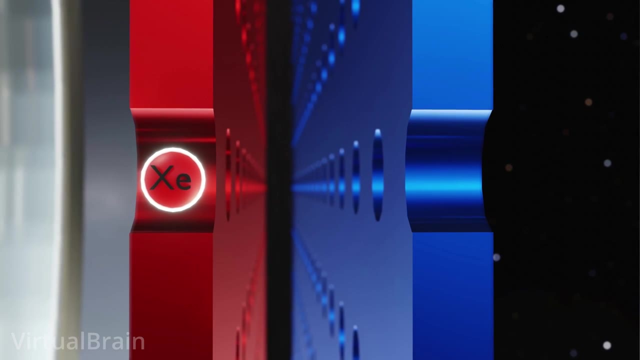 into the container. On the contrary, if we analyze the behavior of xenon, it will be repelled by the first grid. But if we consider that it is being pushed by the pressure of the plasma in the container and it gets through the first grid, it will automatically be repelled. in the opposite, 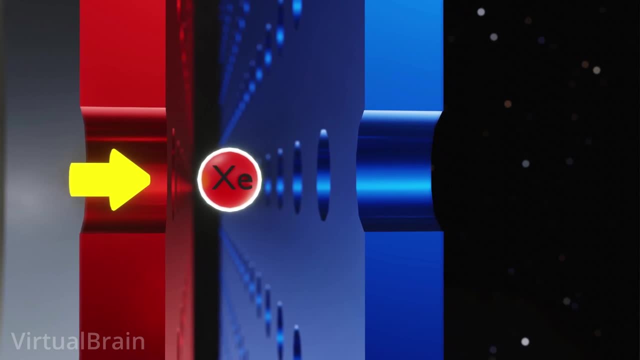 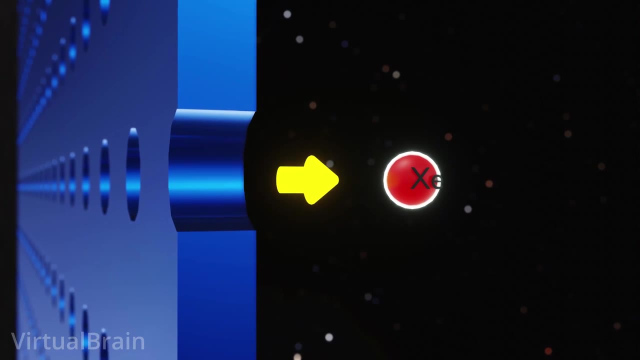 direction. And not only that it will be repelled in the opposite direction, But it will also be attracted by the second negatively charged grid, accelerating the xenon ions to enormous speeds, in the order of tens or even hundreds of kilometers per. 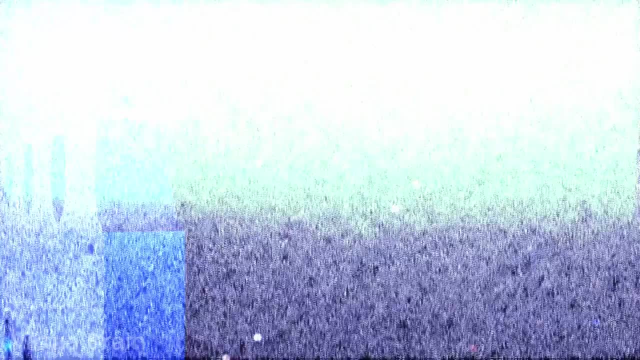 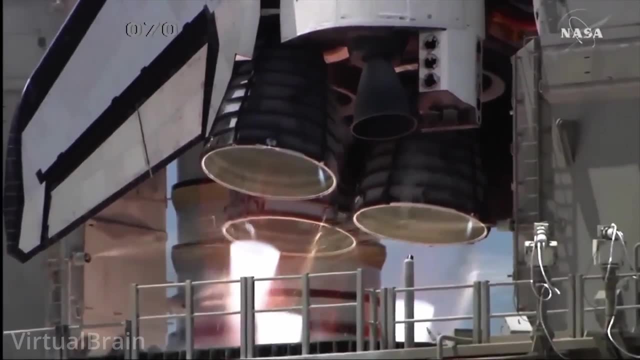 second, depending on the voltages used. To give you a point of reference, the speed at which the gases are ejected in a rocket is only about 3 kilometers per second. Returning now to Newton's third law that I mentioned at the beginning of the video. 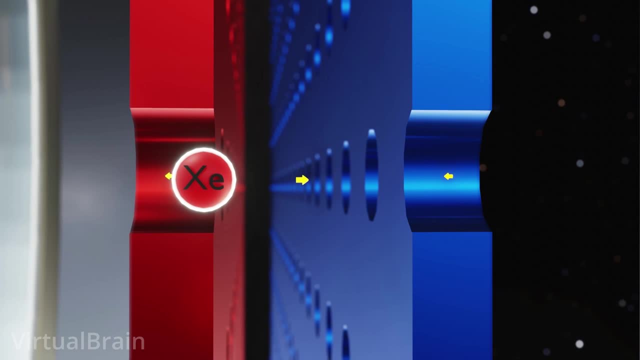 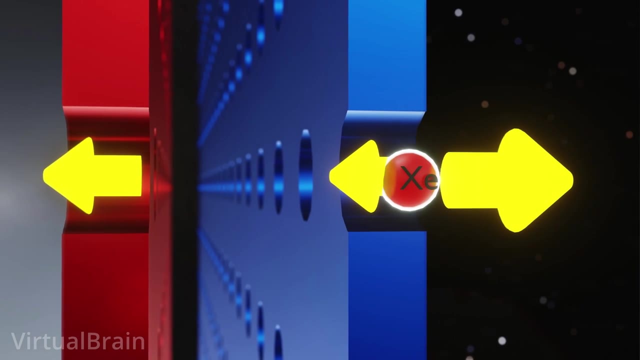 the principle of action and reaction, We will know that the forward-point reaction is the same as the forward-point reaction and that the forward-point reaction is the same as the forward-point reaction. Therefore, if we consider Newton's second law, which tells us that force equals mass, 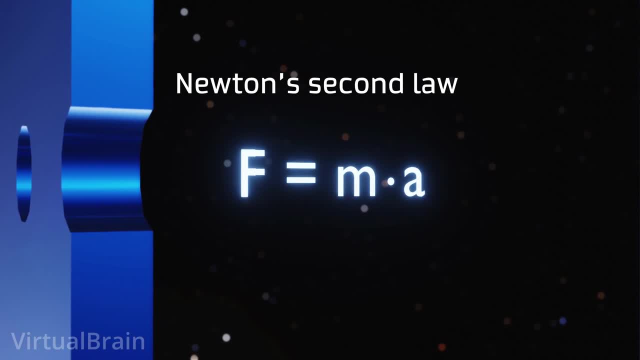 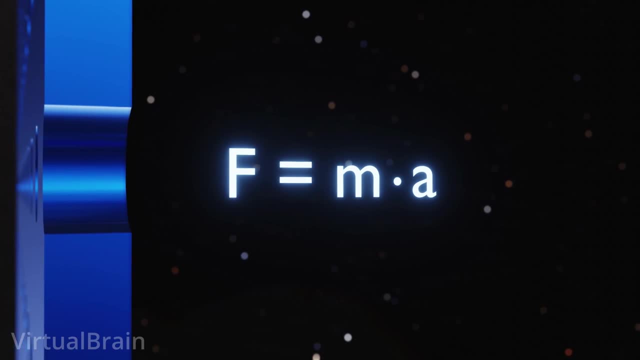 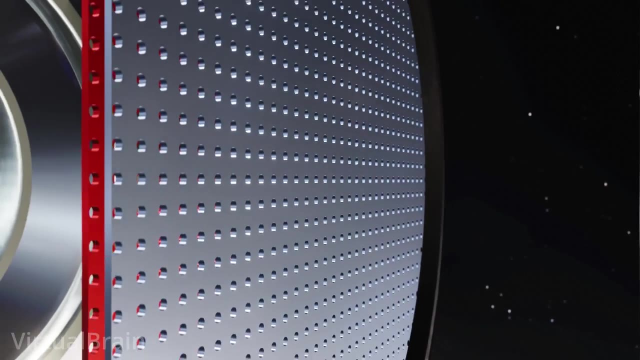 times acceleration. we will realize why the use of gases such as xenon is preferred, because by having a relatively high atomic mass, we are maximizing the two variables that affect the thrust force. At this point, it would appear that we have a fully functional ion thruster, but the truth. 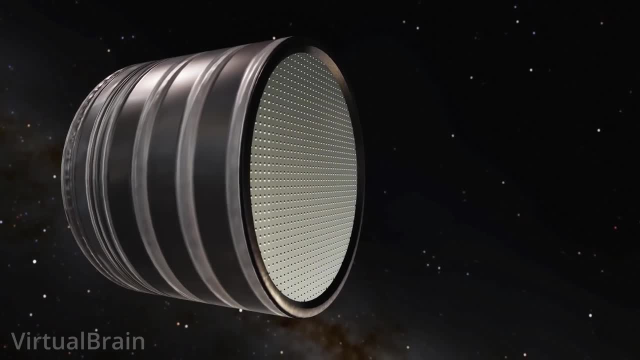 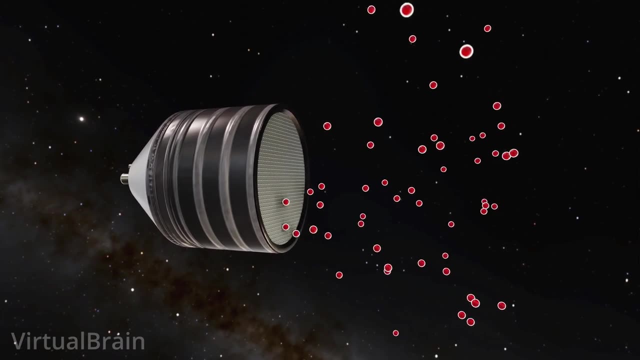 is that we still have a small problem: While the xenon is being accelerated, when it is between the two grids, once it passes through the second grid, the second grid will begin to attract it in the opposite direction, partially neutralizing its effectiveness. 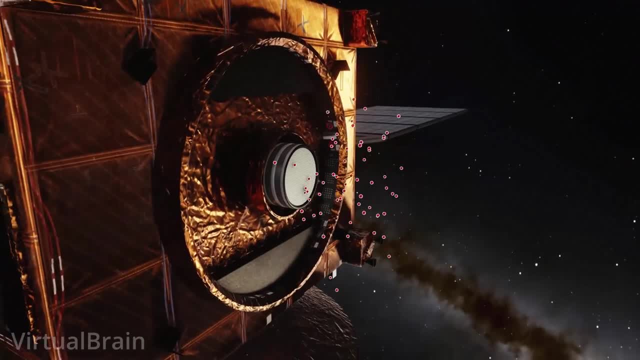 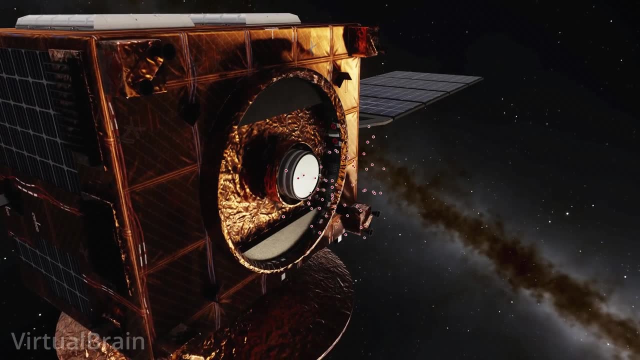 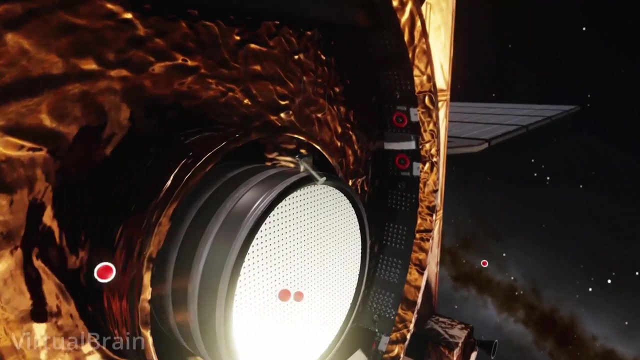 Or xenon ions could even be diverted to other parts of the satellite that might be electrically charged and potentially interfere with its operation. Luckily, the solution is quite simple. The last element is the energy. The last element needed in an ion thruster is a second electron gun on the outside, which 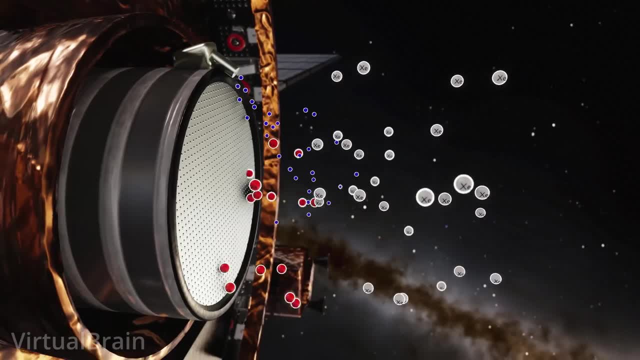 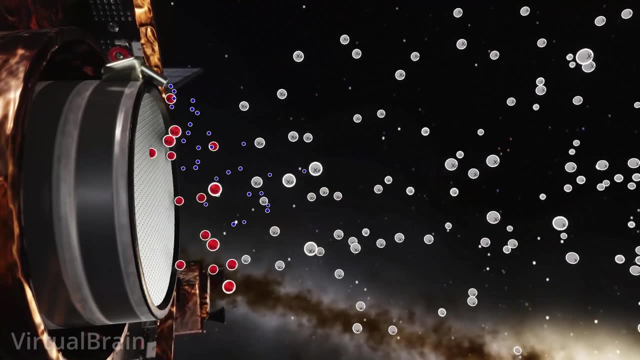 is responsible for returning the xenon ions to a neutral charge, And since the electrons have a much smaller mass than the xenon atoms, their effect on the speed at which they are ejected is minimal. Now that we know how an ion thruster works and that they are capable of ejecting gases,